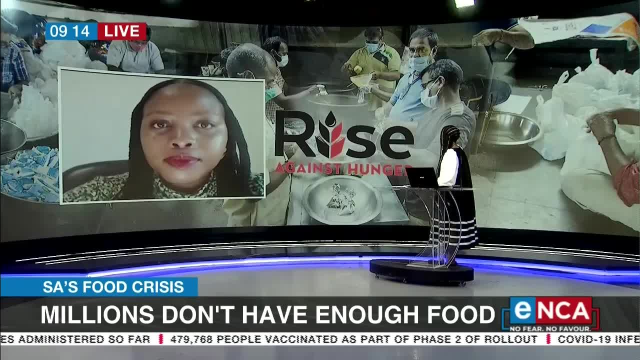 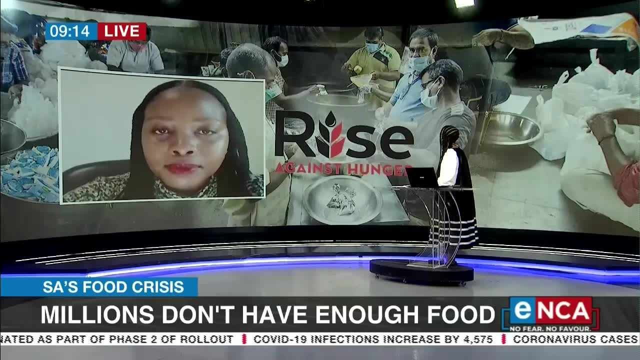 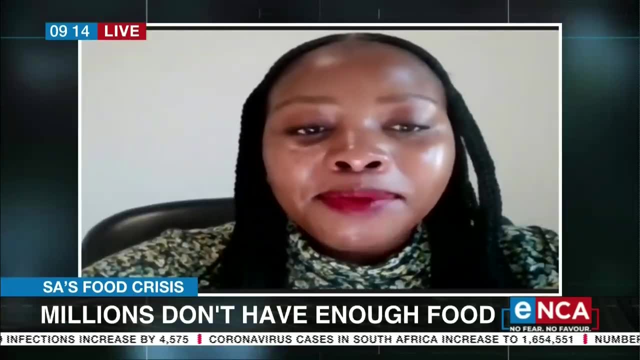 Africa. There are, for instance, foreign nationals and asylum seekers who are here and they, for instance, weren't- they didn't really, especially in the beginning, they weren't- considered for that 350 rand grant. It's more than just us, It's more than just a statistic. I mean, the numbers I'm giving you right now is a sample that was taken. 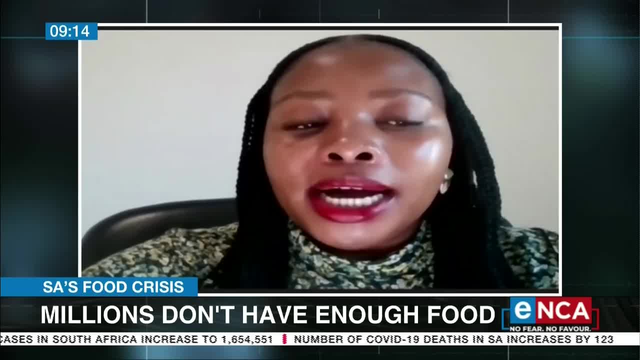 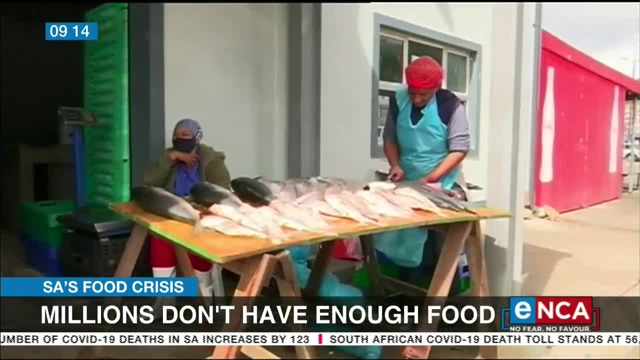 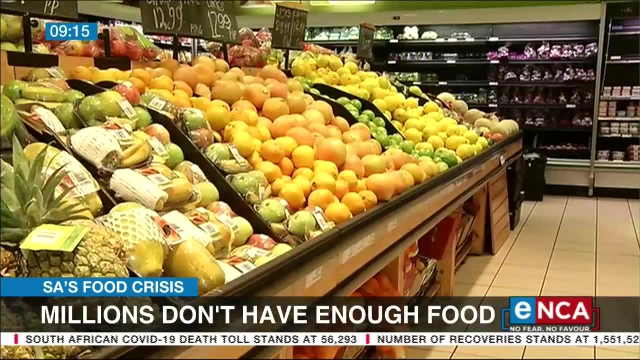 between last year June, you know, in our second lockdown- and up until in March. So those samples is not in fact including everybody else, because the numbers could actually are expected to increase now during the third wave as we speak at the moment. yeah, 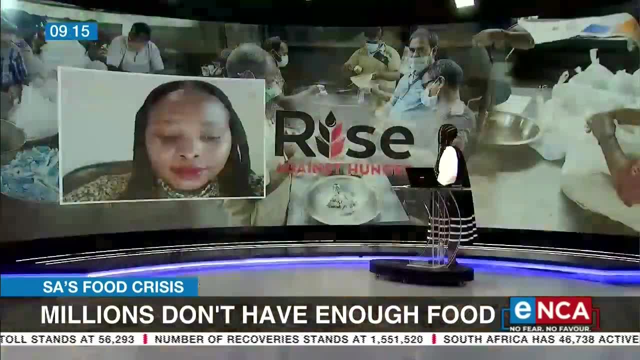 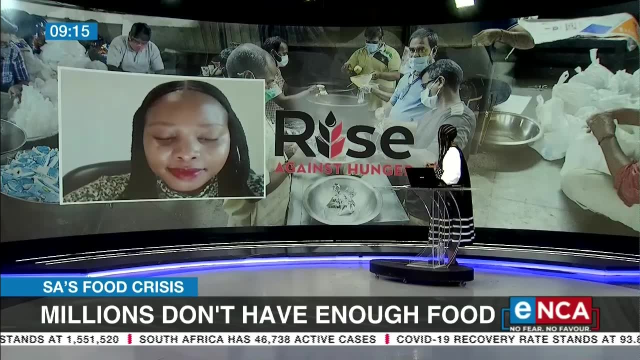 So what do we do? Yeah, What do we do. We know that, for instance, government has feeding schemes. There are some learners, for instance, who literally only rely on that one plate of food that they get during break at school. So we know that the government has 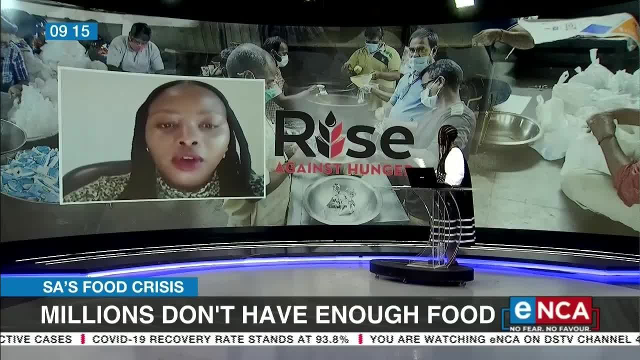 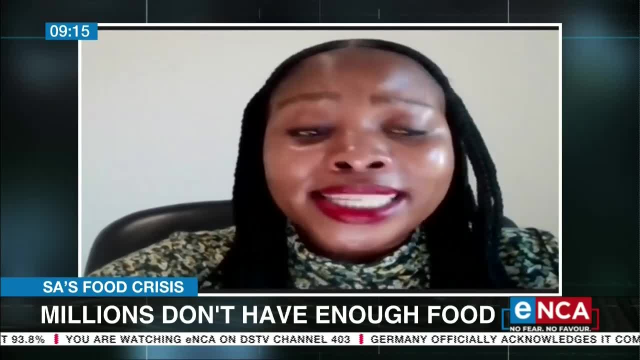 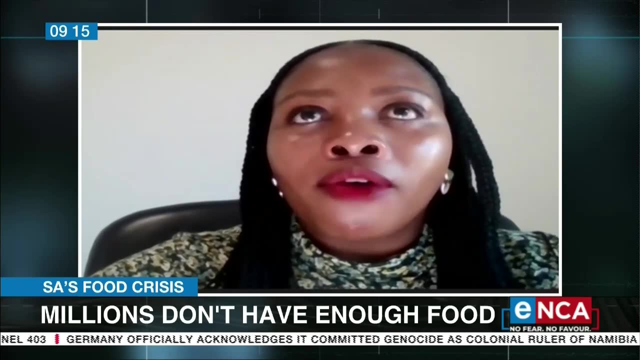 a constitutional obligation as well. But what do we do? Of course, Because the private sector also has to step in. You know what? I think it's all sectors that need to step in, But I think what has happened really during this period is that, you know, it has highlighted the dysfunctionality in our food. 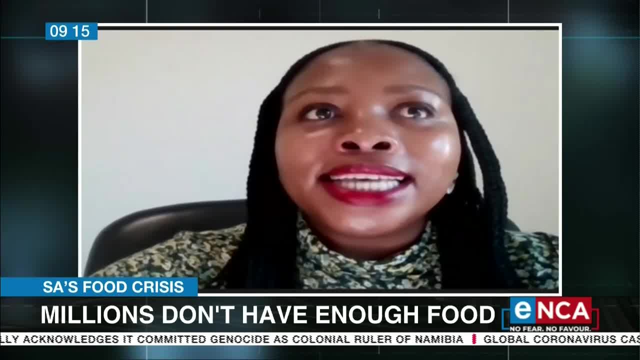 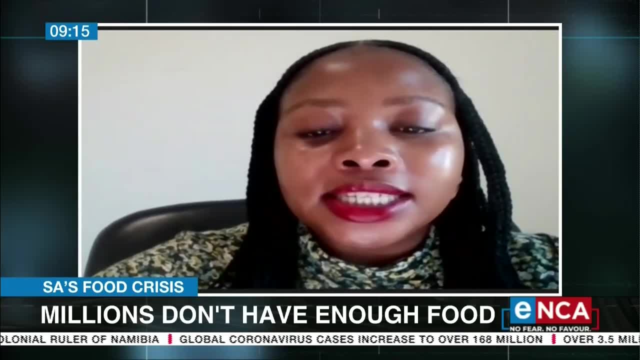 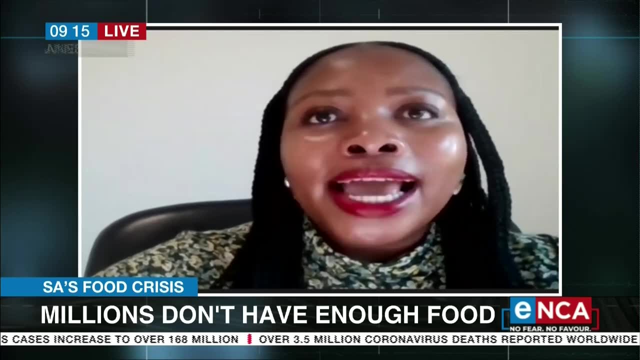 systems and in our health systems. And I think what this has done is, basically, it has given us an opportunity to look at, you know, our opportunities within, you know, like within our agricultural sectors. It has given us an opportunity to look at our nutrition care systems that they not only just focused on, you know, treating the 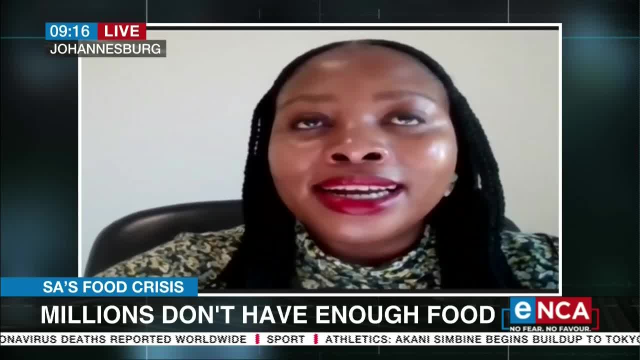 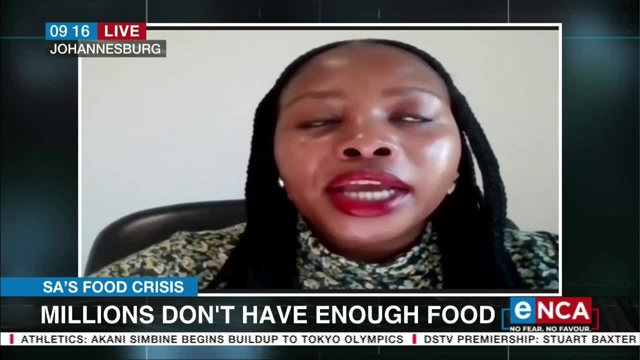 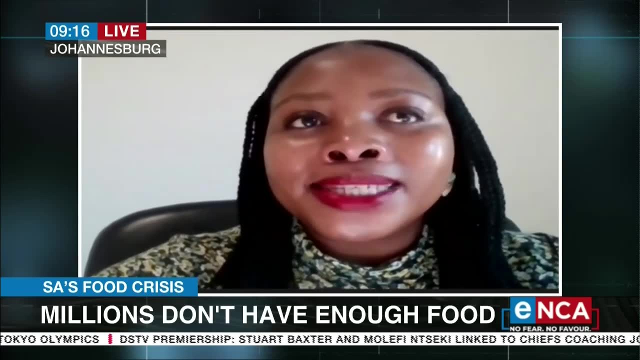 problem. but actually, how do we integrate nutrition into those systems? Because, Masiho, the access to food it's not, you know, it's not simply a choice, you know, for civilians, but basically it's hindered by, you know, systems and structures and living conditions you know around. So it's a human, you know it's a human. 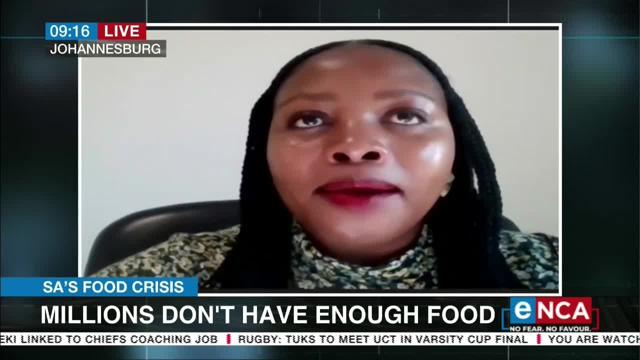 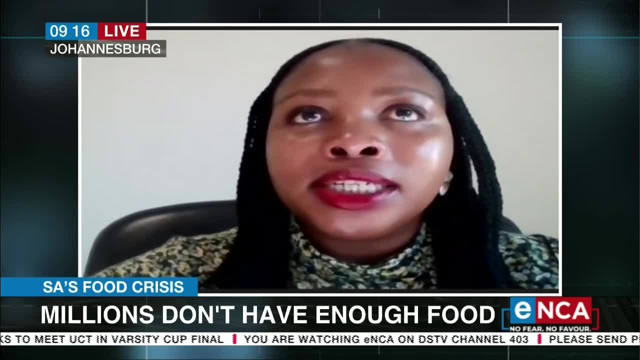 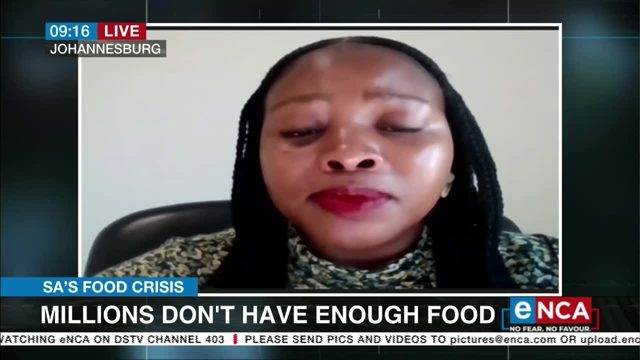 right, but in addition, it's an equity and it's an equity problem. So you know, it has to be addressed within the food environment. But I also think that there is an opportunity. There is an opportunity here to also, you know, affect the health, I mean the health systems as well. 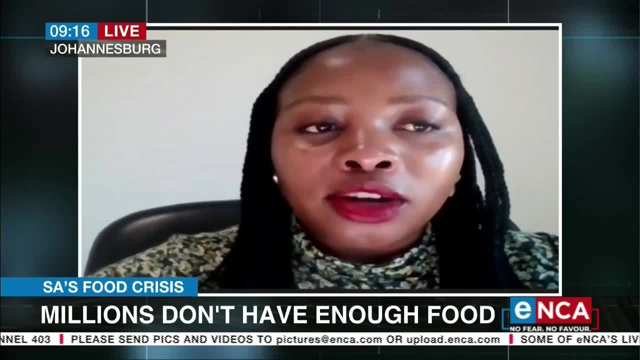 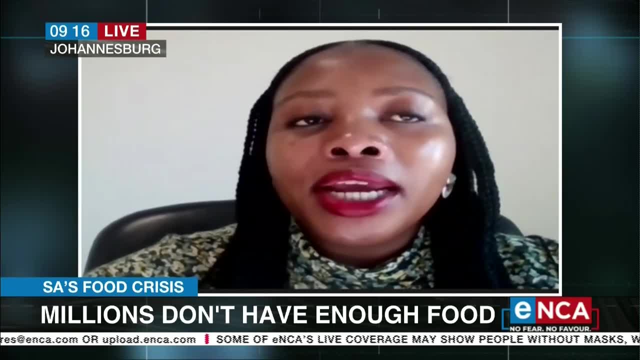 Because, you know, within the years, besides just looking at COVID-19 right now, within the years what we have discovered is there has been a quite a very- you know- increased rise of you know undernourishment. 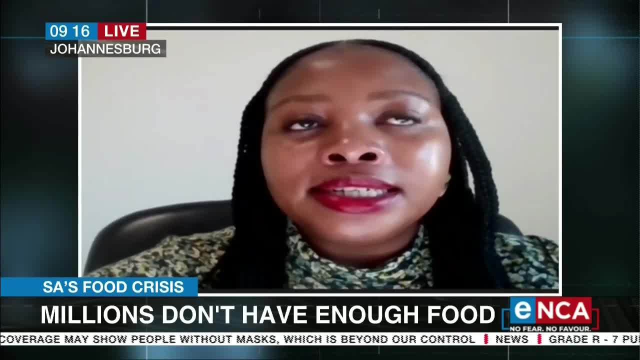 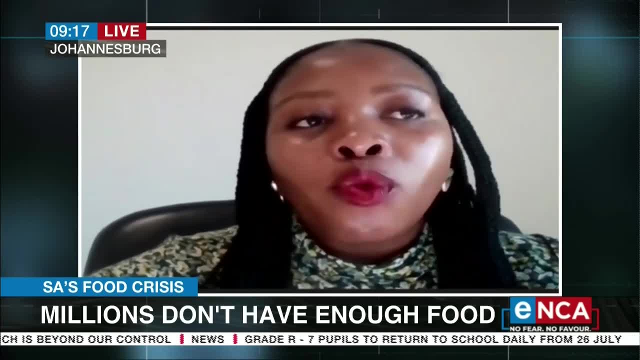 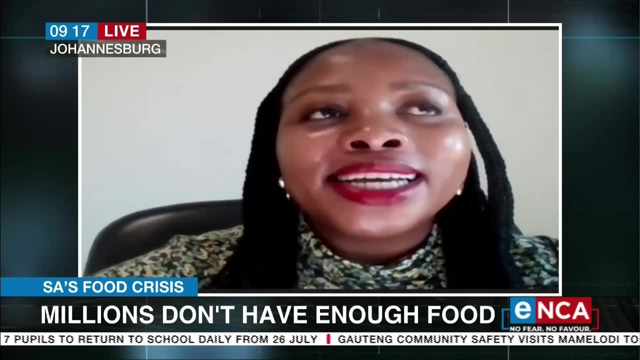 But then you also have, you know, issues like diabetes, you know, like the non-communicable diseases arising from dietary barriers. So you know there's a lot of, you know, health-based issues, And what we've sort of done as a country is that we have, you know, directed a lot of budget towards the medical 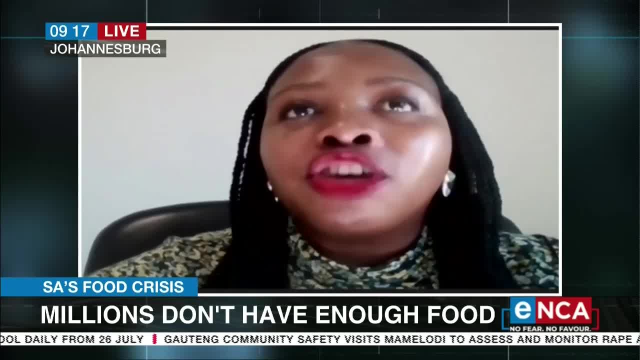 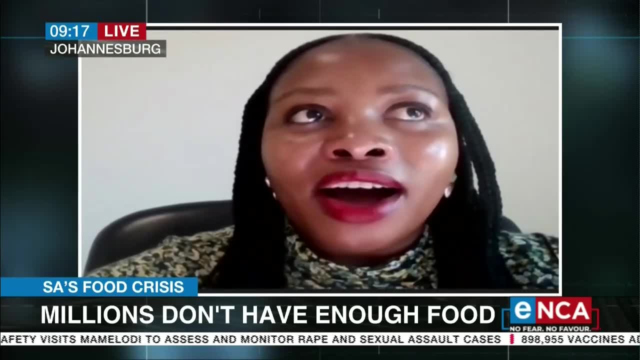 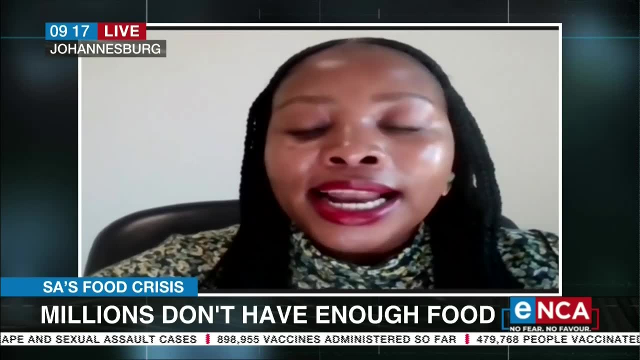 attention in treating those, instead of actually looking at acute preventative measures that enable people to strive where they work, where they play, where they live in environments, you know, like preventative measures that enable people to be able to strive. So it's not only just literally the, you know, like the factor of you know, having, you know, a health care system. 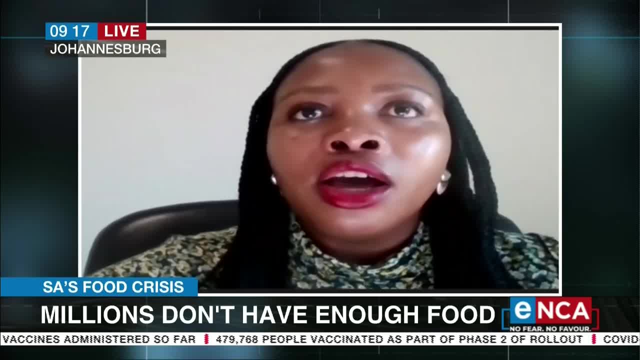 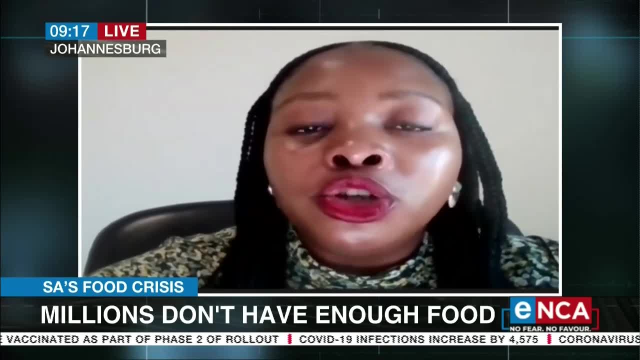 of, you know, having food availability, but it's having food access, it's having food availability, it's having food affordability, you know, and it's also having the infrastructure being conducive, you know, for civilians to be able, you know, to provide for their families and for themselves. 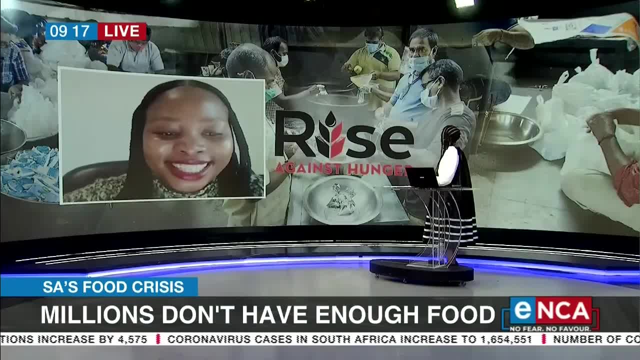 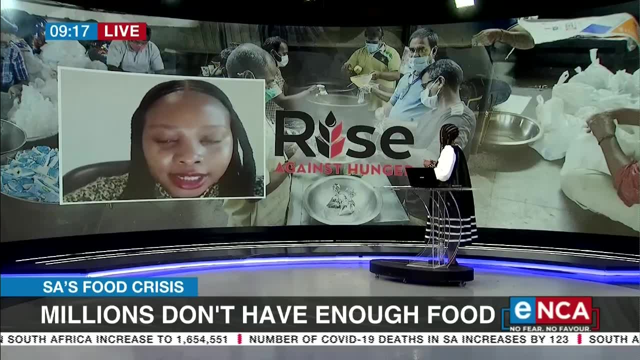 And I mean I'm sorry, my voice is, my voice is so bad. That's okay. That's okay, Let me not strain it for too long. but I just have another question and I'm sorry for roping you into this, you know. 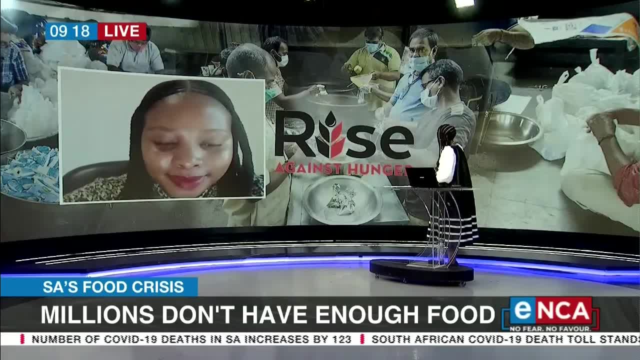 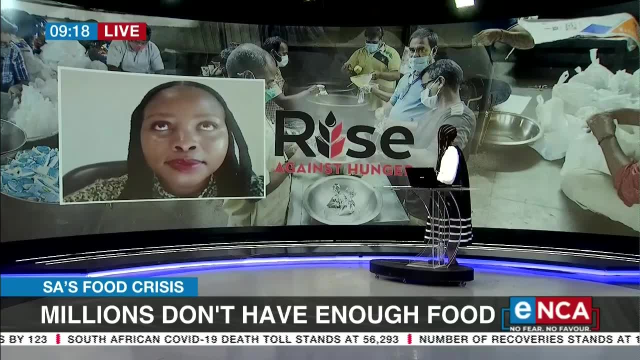 the emergency, the corruption issue, The corruption emergency that is happening in South Africa. This is not just government, of course. There are enablers in the private sector, who are the bribers, and government, obviously, some people being found wanting. 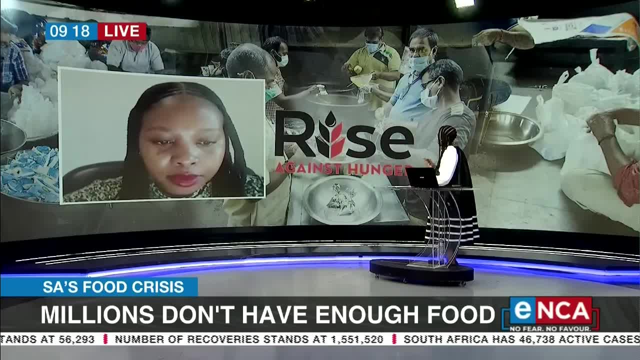 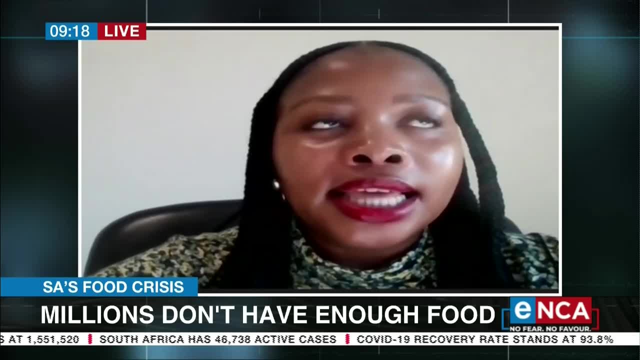 That is also something very disappointing that could be used. that money could be used to eradicate hunger in the country. You know I'm going to speak in the sector of hunger and nutrition because of course, you know most of our work for 43 years. 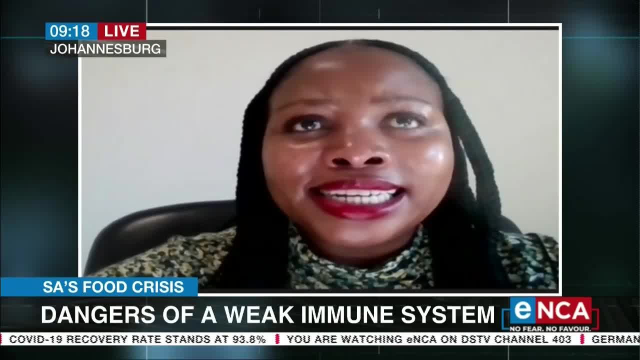 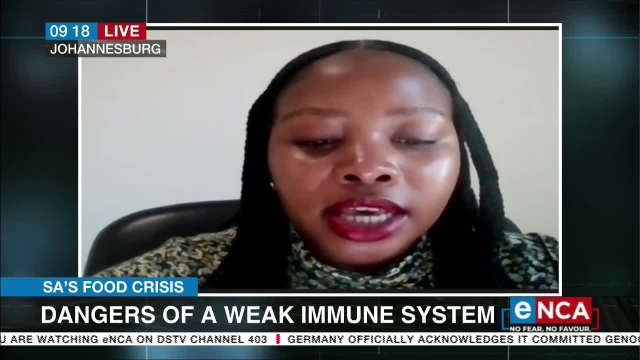 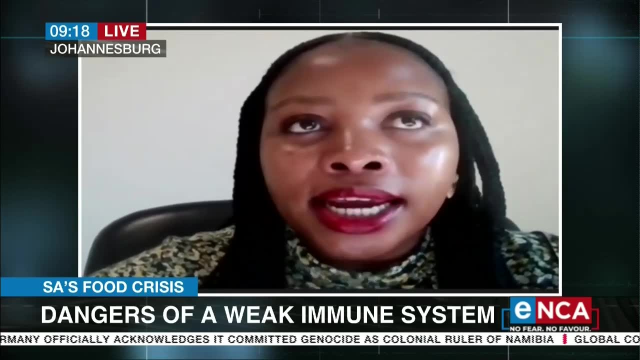 has been concentrated in this And I think, with the understanding that government, you know, and other food actors are generally just favor interventions, you know that are on an individual level efforts, I think if we were to look at an inclusive and a pro-equity, you know- approach, you know some of those problems can be because 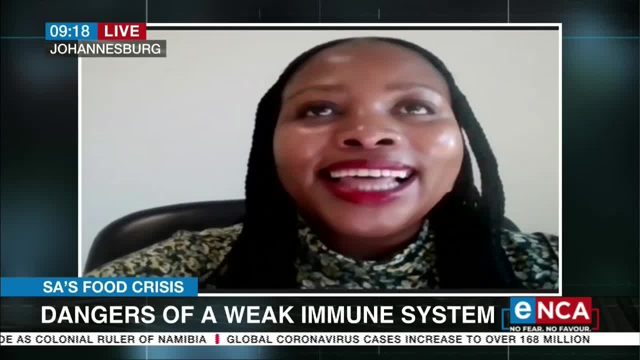 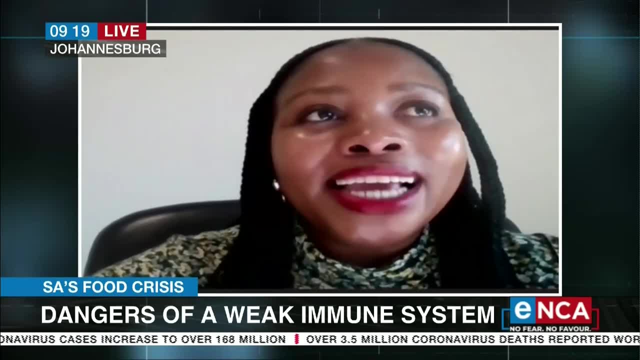 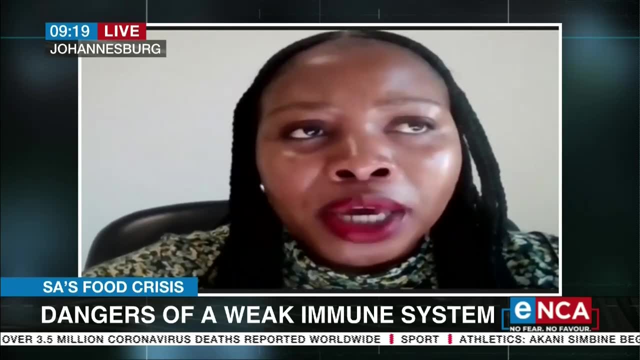 you know if we've got proper investment policies that enable for accountability. you know if we hold policies that account. you know food and beverage- If we hold policies that are actually beneficial to the people and the industries and how they promote. you know. 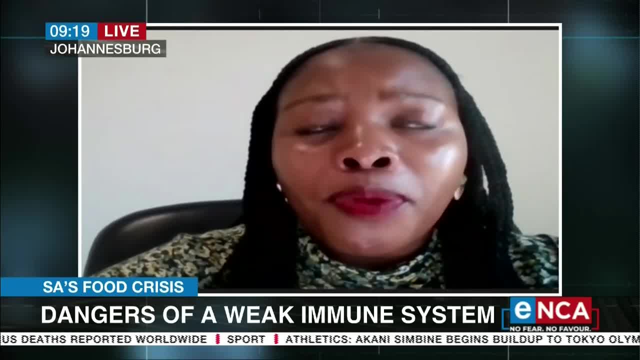 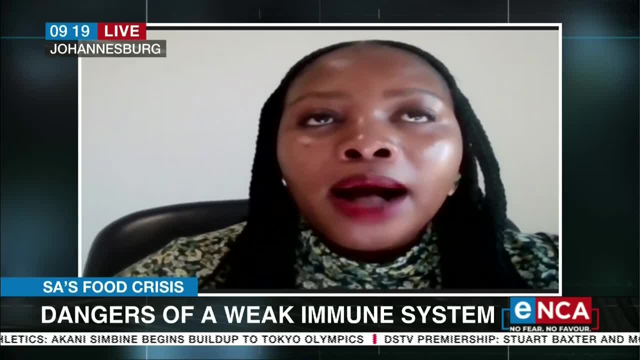 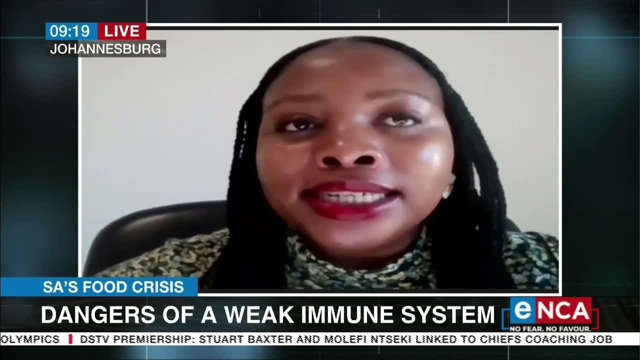 like you know, healthy diet and make them accessible to people you know that would also assist. I mean you know Masihua. over the past 11 months we have seen an increase on staple crops for food prices increased between 30% to 147%. 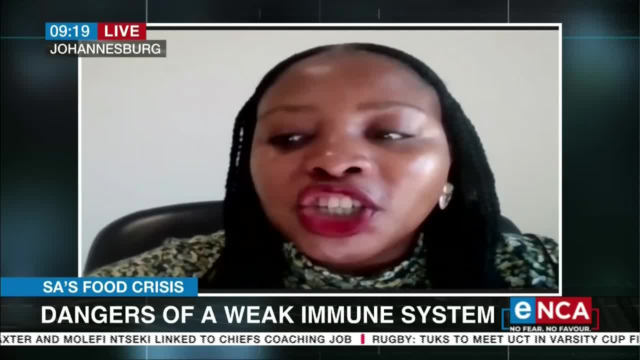 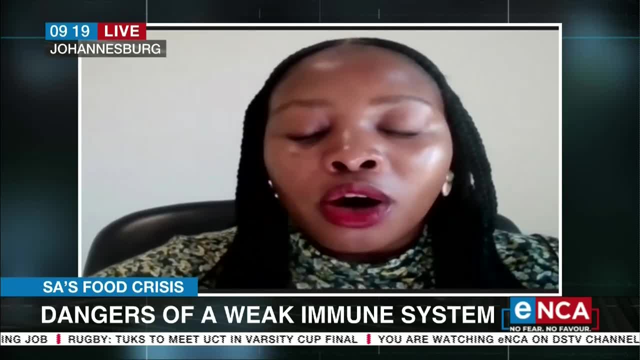 And this is dependent, you know, on availability of the crops and also on the food market, And this is dependent on the seasonal crops. And this shouldn't happen because we were promised, prior to the you know, prior to the, you know to the lockdown, that the commission's price commission is going to be stepping in and looking at these types of corruptions. 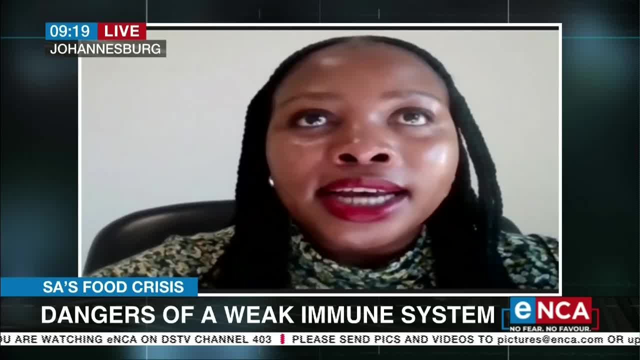 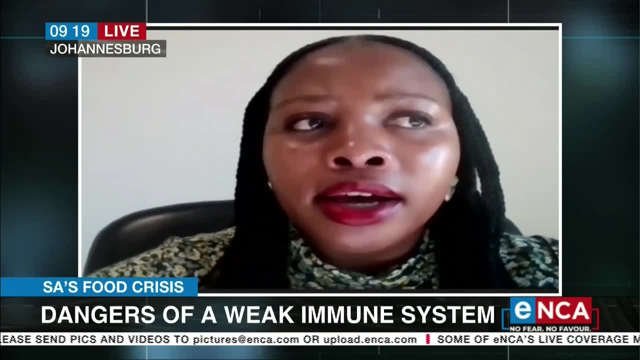 So we've got all of those agencies that needs to be looked at. I mean, we've got also opportunities where we need to hold, you know, you know, the private sector accountable to ensure that they give back, you know, to communities where they operate in. 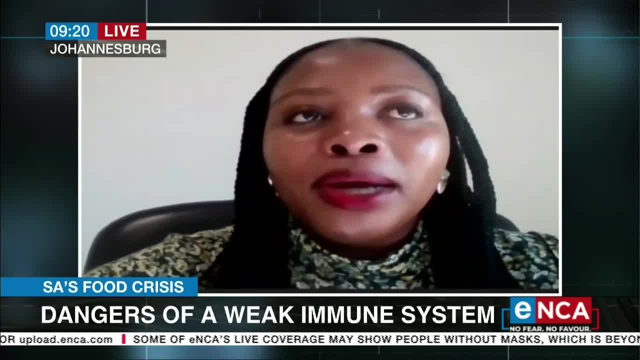 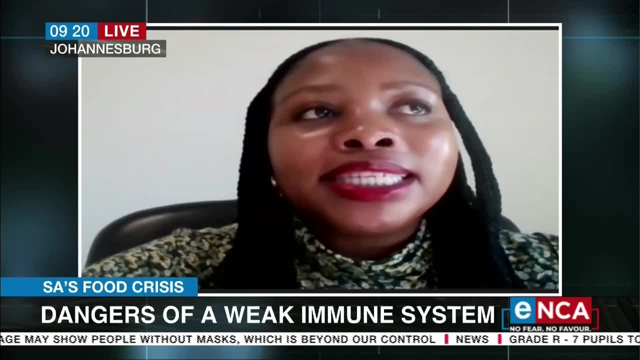 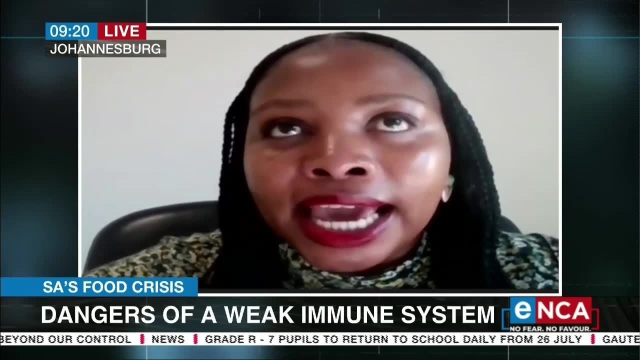 And who is actually? you know. I mean, the private sector is the private sector. The private sector is doing so far, But you know, like things like minimum wage being addressed and actually being monitored. you know things like CSI BEE, you know. you know like seeing them being implemented and being forced on a larger scale. 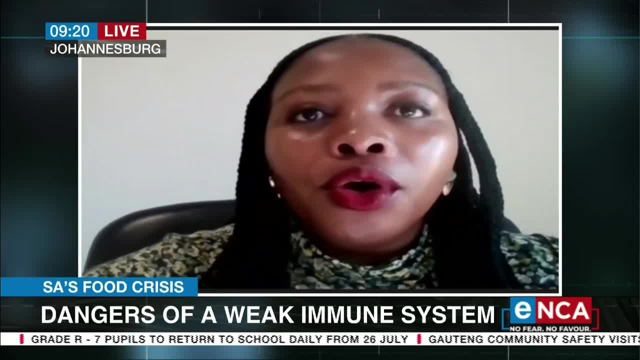 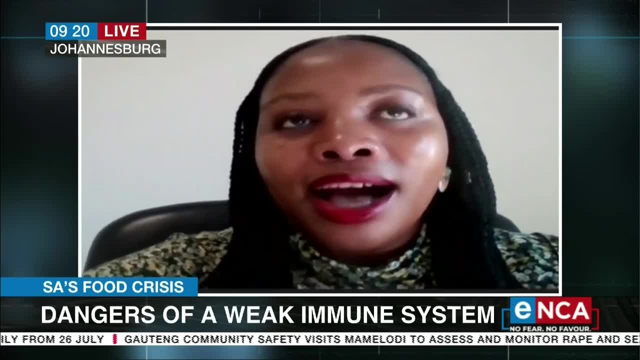 Those are the things that can be immediate resolutes, you know, within the country, without us actually having to look at you know, like really trusting measures, But we need to look at sustainability, accountability, investment being actually addressed and going down. 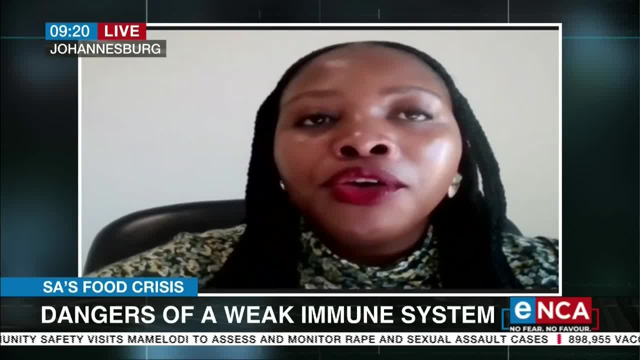 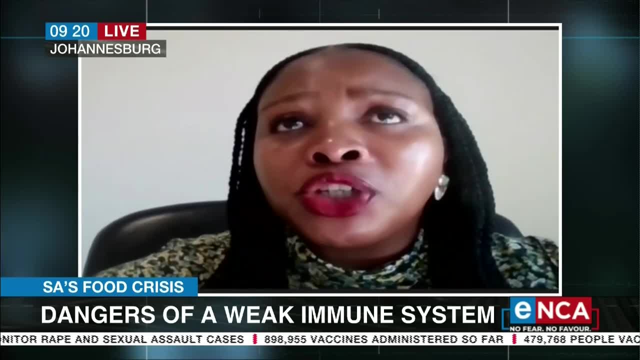 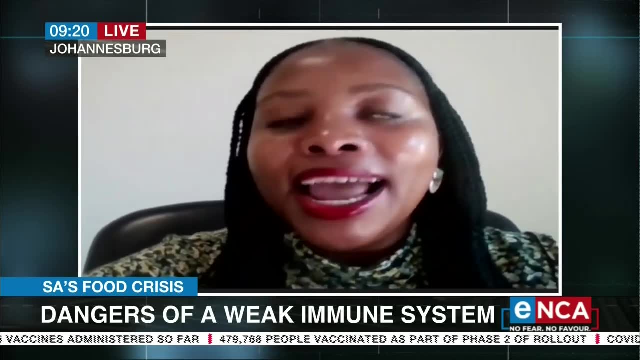 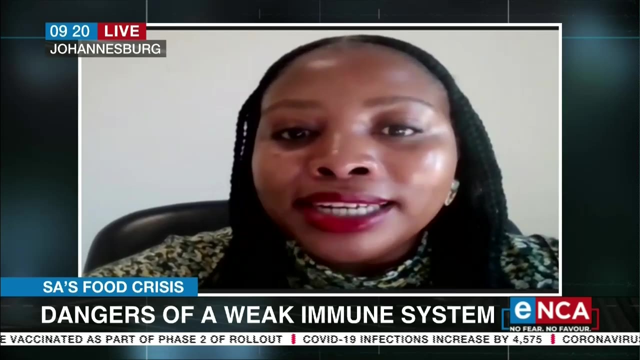 Right And also, just, you know what is the distribution of equity across opportunities across. you know, like the entire supply chain to ensure that the people at the bottom of the pyramid actually have good access. you know, And the models enable them not to be so much dependent but to be actively involved. you know, in transforming. you know, like the economy, the environment. 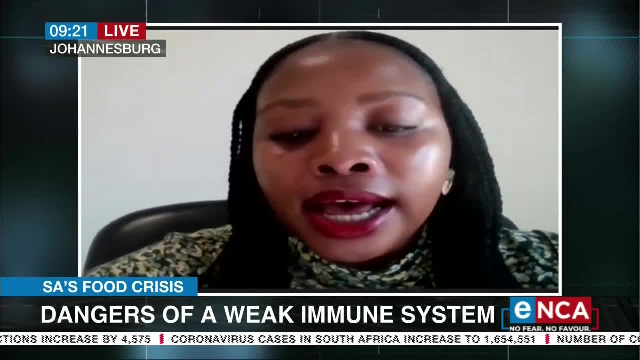 Right And also our social, our social issues.